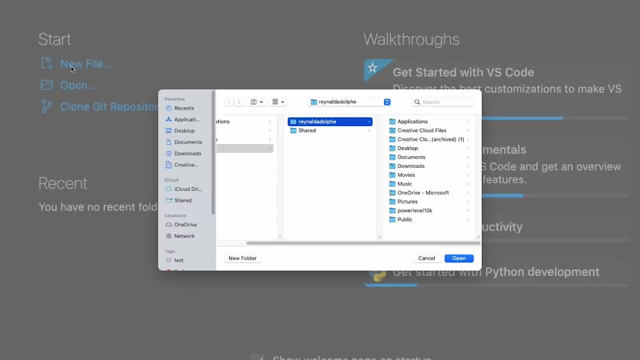 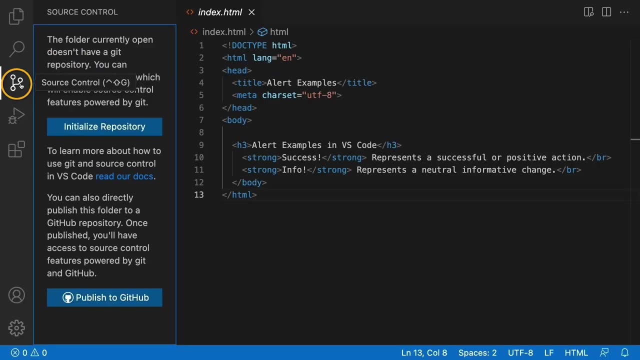 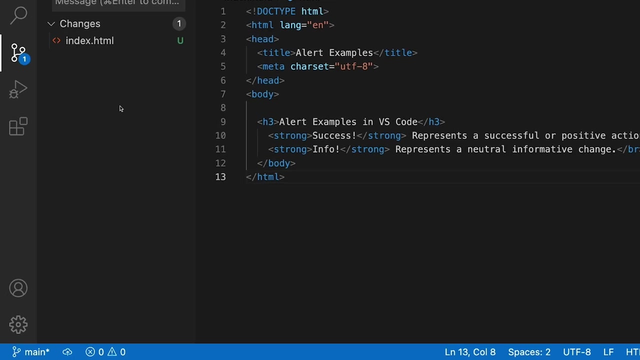 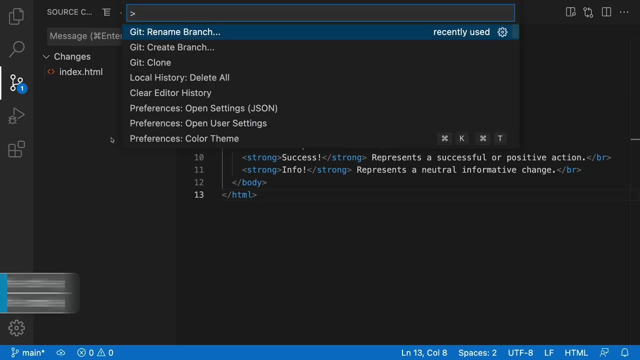 is to initialize a folder to reflect your repository. So let me open up an existing folder with some files in it and then go to source control and click initialize repository. Now notice at the bottom left hand corner that the branch is named main. but if you needed to rename it you can simply open the command palette shift. 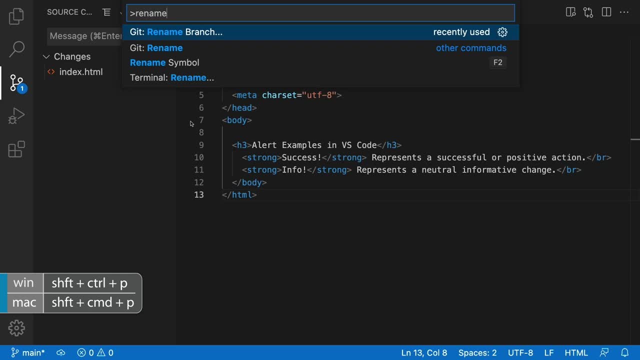 command P and type rename. and let's say we want to call a test branch and just hit enter, and now you see it reflected below, but I'm going to rename it back just as easily to main. Now, after initialization, you'll see that in the source control panel that my new file shows up with 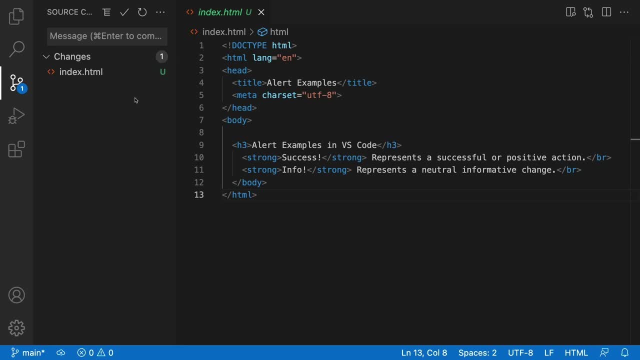 the letter U beside it. So I'm going to rename it back to main and I'm going to rename it back to U. beside it and U stands for untracked file, meaning a file that is new or changed but has not been added to the repository. So to track it I can just click the plus sign next to the indexhtml. 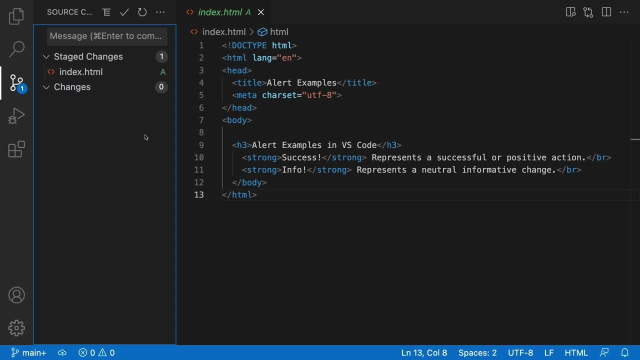 and now it is what's referred to as staged. Now, once added, the letter next to the file will change to A, which represents a new file has been added to the repository And the next step would be to commit it, and all I need to do is add a message such as: first commit and then I'm going to add a. 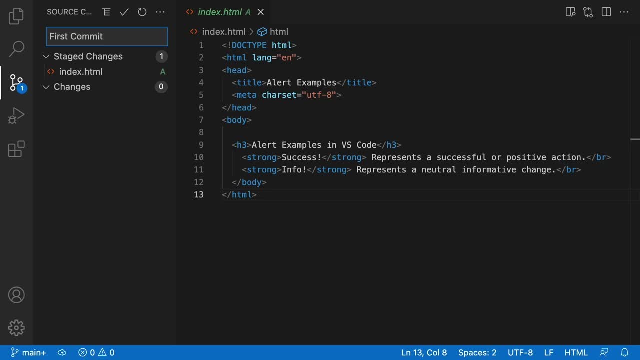 message that says commit and in general it will just describe whatever change that you make. it's for informational purposes and to submit it, I'll just hit the check mark right above it. So right now we're on our main branch. but if this is a real application and we need to add new code, new. 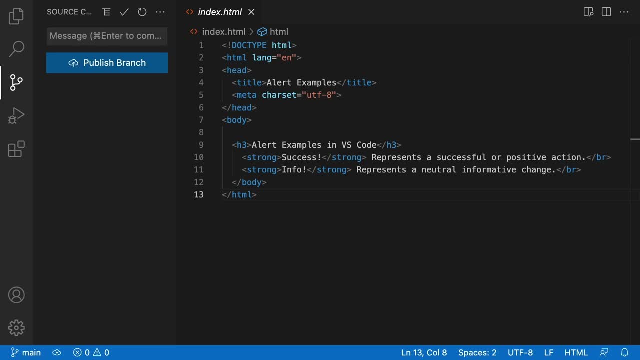 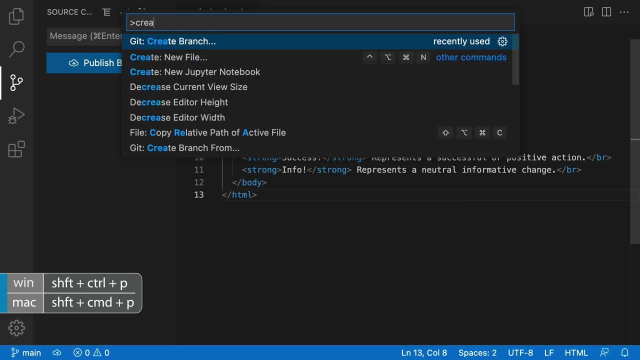 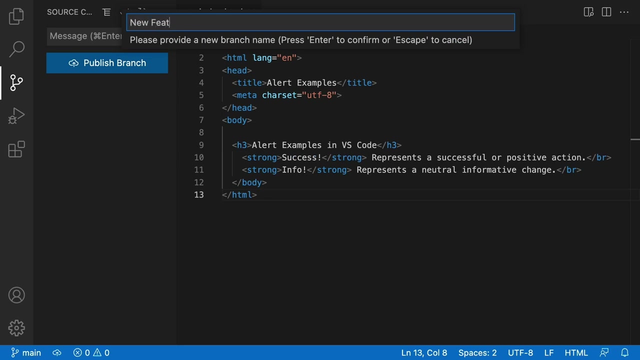 features. for example, we want to create a separate branch. to do that by going to the command palette, shift command P, and I already have the option here to create branch. but you could also just start typing in create branch. I'll call this new features and the bottom left hand corner reflects that now, and I'll add two lines of code that. 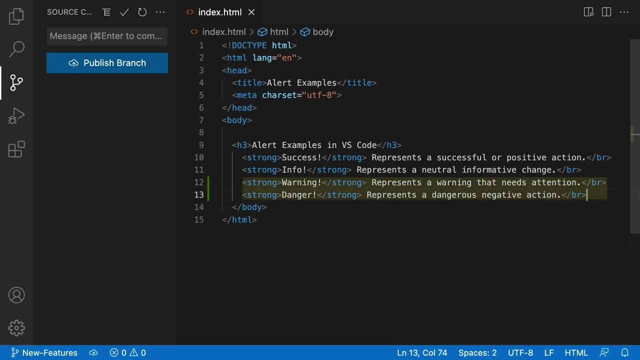 reflects my new features, One for warning and one for danger. Now you'll notice when I add the code. on the left hand side there's this area called gutter. for new lines of data, it's reflected by a green line. for changed lines of data, it's reflected by a shaded blue line. 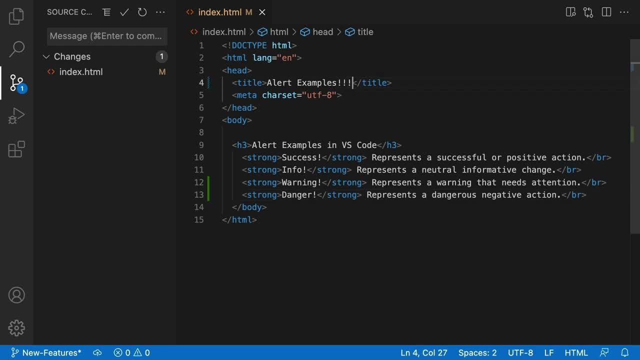 So let's say, if I added exclamation points on line four, you'll see a shaded blue line, and if I deleted a line like line 10, it'll be reflected by a red arrow. but I'm going to put that line back Now, right under the 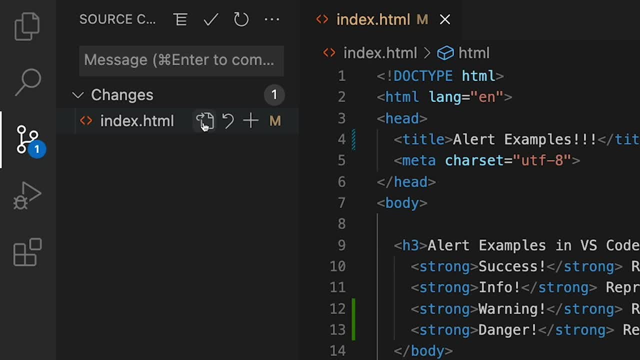 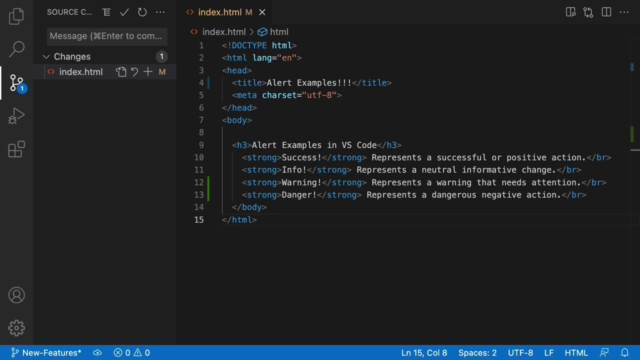 word changes. you'll see I have some icons here to open a file, discard changes that I've made. I can stage my changes and this is all for one file. but if I had multiple files, then I can go ahead and discard all my changes or stage all my changes. Now Visual Studio Code also has the ability to perform a diff on files to compare files side by side. 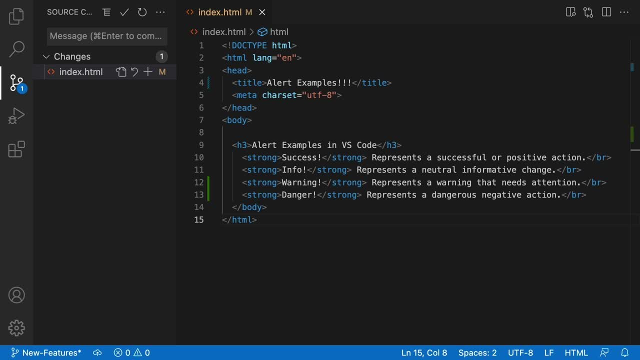 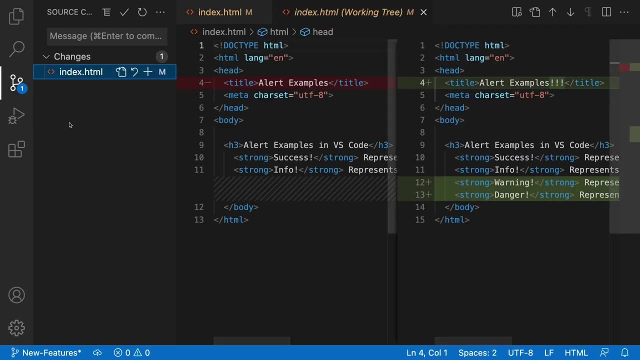 Typically you would need to have a separate tool to do this, but it's built in, and to see our changes side by side we just need to click on our file. But this time I also want to show you that you can see all the changes in one file. So if we go to the upper right hand corner here, 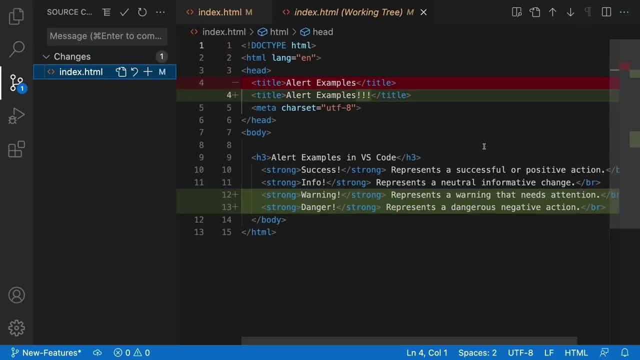 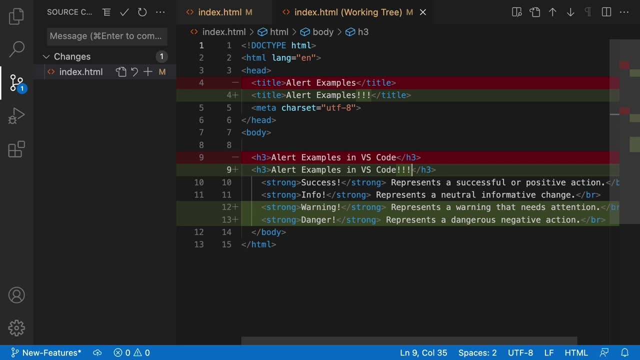 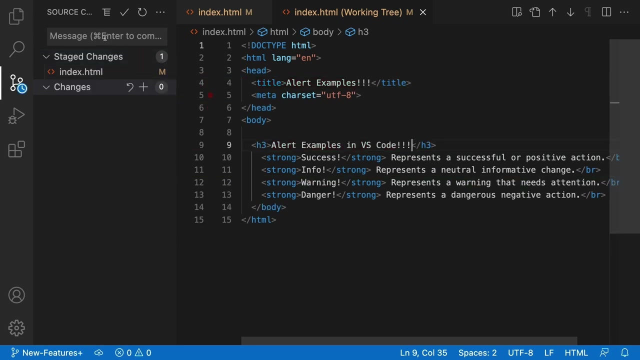 And choose inline view. it consolidates them And within here we can also make changes. so I can add some exclamation points here if I wanted. So now, if I want to stage my changes, I could come up here and click the plus sign and add a message: call: added features and committed. 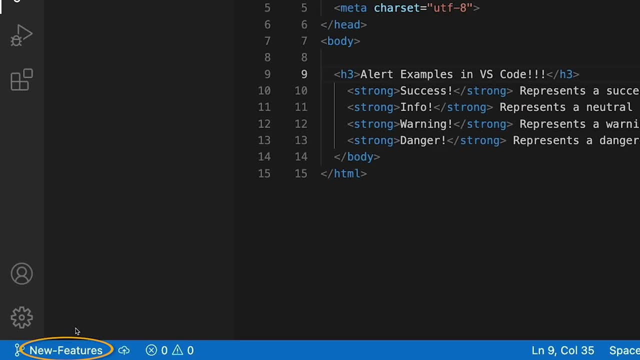 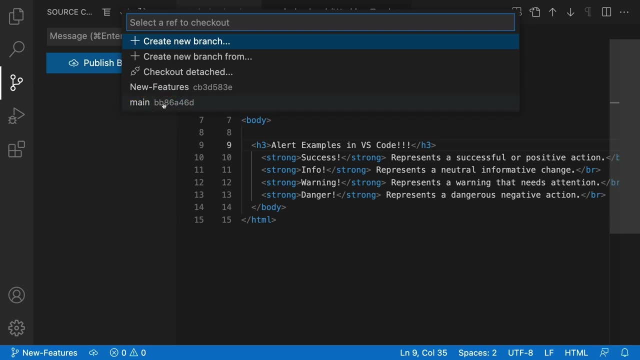 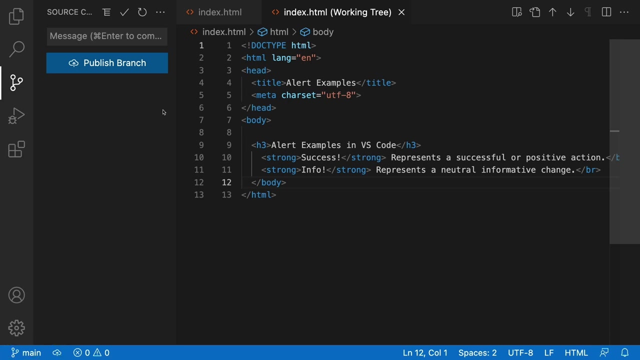 And remember now, at the bottom left hand corner it still says new features and that's the only branch that's affected. So I can click here And switch to main branch, And this is how the code was originally. Now, if I want the new code to be reflected in the main branch, I need to merge. 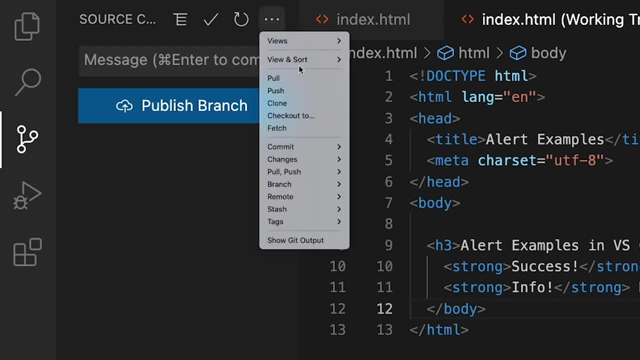 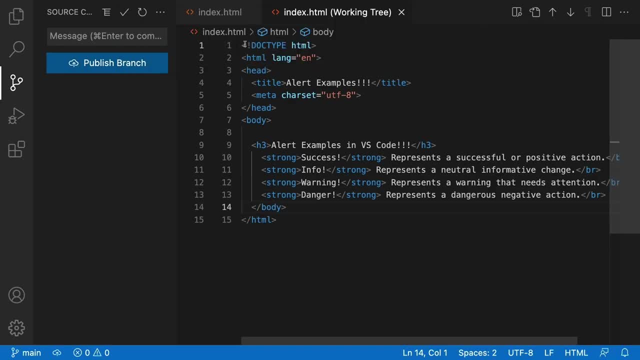 By going to these three dots here, Going to branch, Merge branch- It'll ask me from where? And I want to select from our new features- branch. And now our main branch has the reflected changes. So now let's say we actually want to publish this to Google. 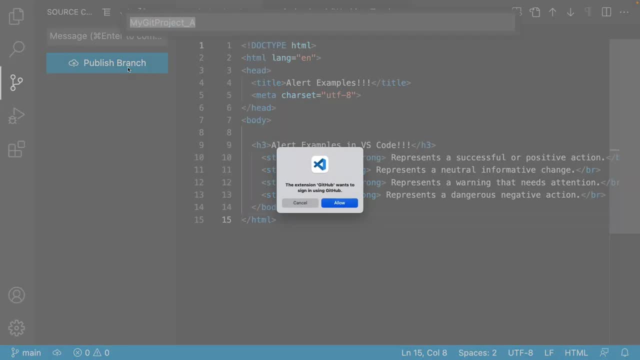 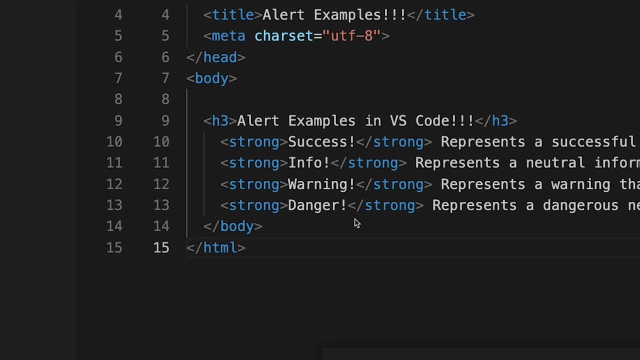 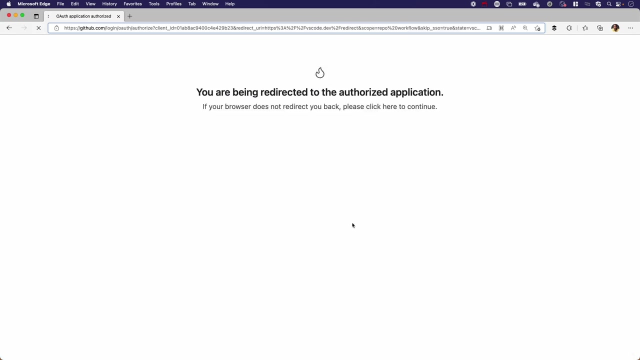 Or to GitHub. All we need to do is go to publish branch. It's going to prompt us that this extension GitHub wants to sign in using GitHub. I'll hit allow And then an authentication process will start. I'll hit continue at this prompt.